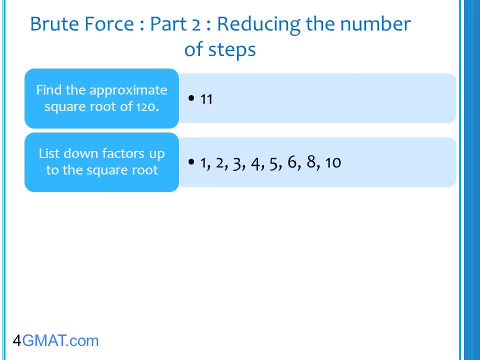 Allez. Factors up to 11, that are, factors of 120, are 1,, 2,, 3,, 4,, 5,, 6,, 8 and 10.. Count these factors. you have a total of 8 factors up to the square root. 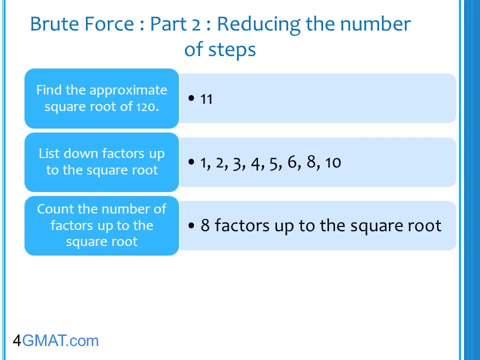 The last step is where we find the answer. If a number has got 8 factors up to its square root, it will have 8 more factors between its square root and the number itself. So if 120 has got 8 factors up to the square root, 120 will have a total of 16 factors. 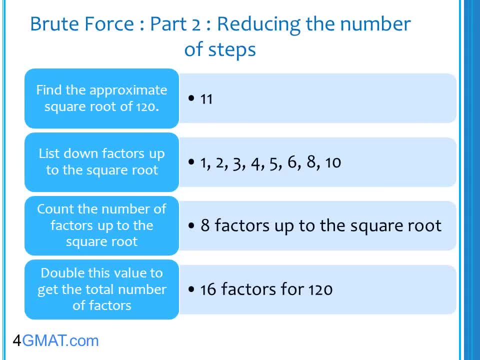 All you need to do is simply double the number of factors that you have found till the square root of the number. This method works as long as this number, 120, is not a perfect square 120, for instance, if you look at a number like 36,. the method needs a slight alteration. Try it out. 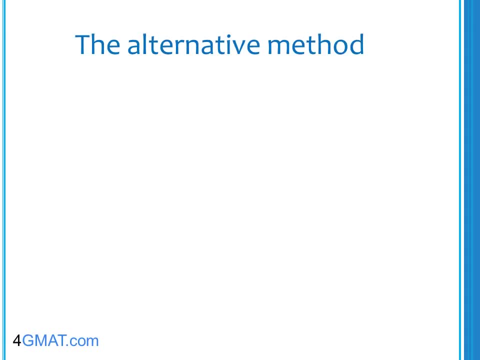 The third method does not use any of these. The third method uses brute force. It is an elegant method. It is a three-step process. The first step: express the given number as a product of its prime factors. 120 can be expressed as: 2 cubed into 3, into 5.. 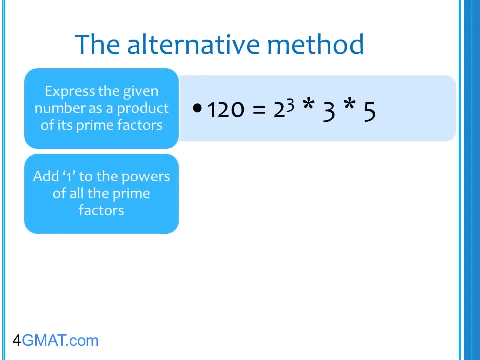 Add 1 to the powers of all of these prime factors. The power of the first prime factor, 2, is 3.. Add 1 to it. The power of the second prime factor, 3, is 1.. Add 1 to it. 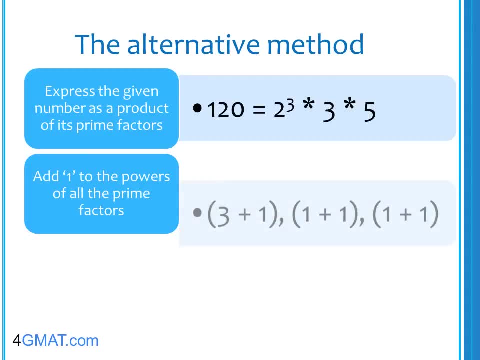 And power of the third prime factor. 5 is also 1.. Add 1 to it. What we have is 3 plus 1, 1 plus 1 and 1 plus 1.. The third step gives us the answer. Multiply the result in step 2, which is 4 into 2, into 2.. 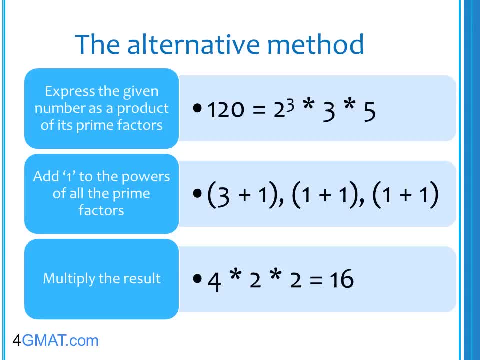 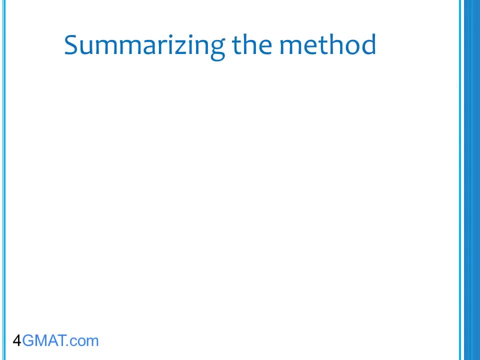 16 is the total number of factors. that 120 has Any error that one would have made. by missing out a factor is completely eliminated in this. 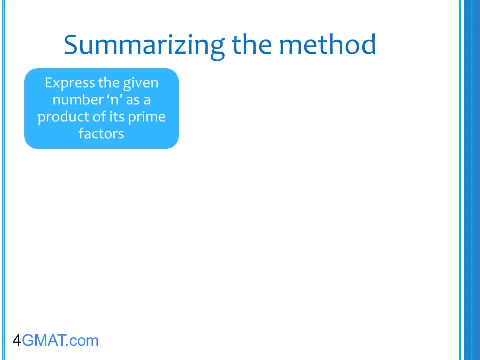 I'll summarize this method. The first step: express the given number for which we are finding out the number of factors as a product of its prime factors. Let's say n is equal to a power p into b power q into c power r.